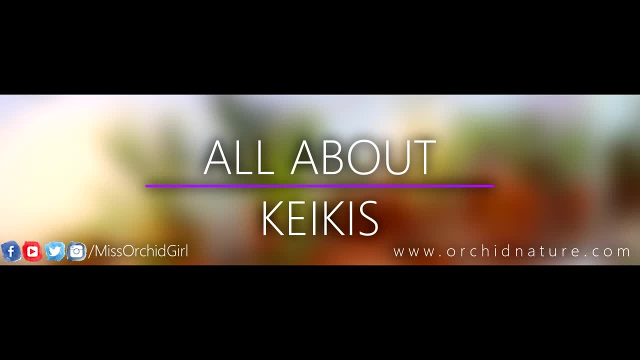 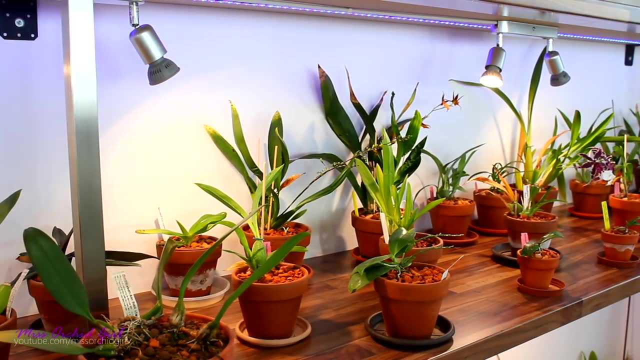 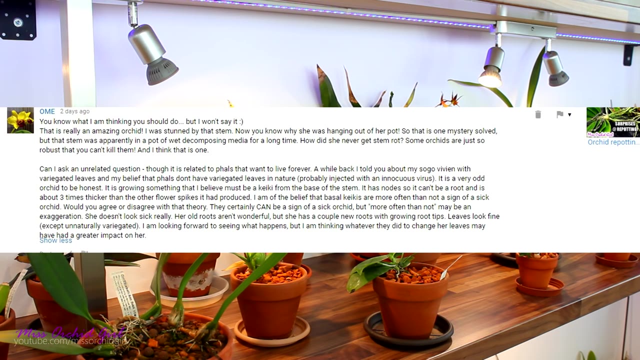 Hey guys, it's Dani. Today we're gonna discuss about orchid cakies. We're gonna turn the subject inside out, and this is because one of my viewers asked me if stress is the only reason why orchids produce cakies, And then I asked you guys if you'd like a video debate on it. You said yes, Therefore. 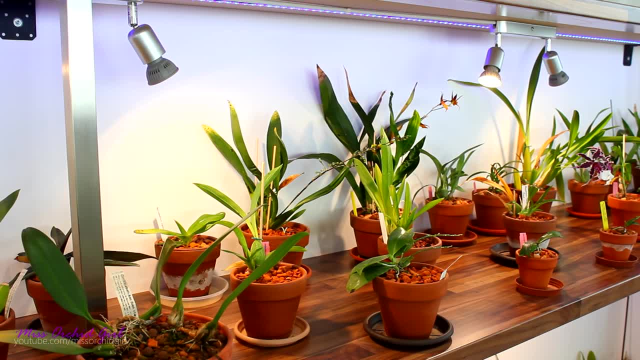 this makes it a video request, and that's what we're gonna talk about. So the way I structured this video is to have a more factual view and also a more theoretical view, And if you know me, you know I love these discussions. Okay, let's get to work Now, because I do have a video in which I 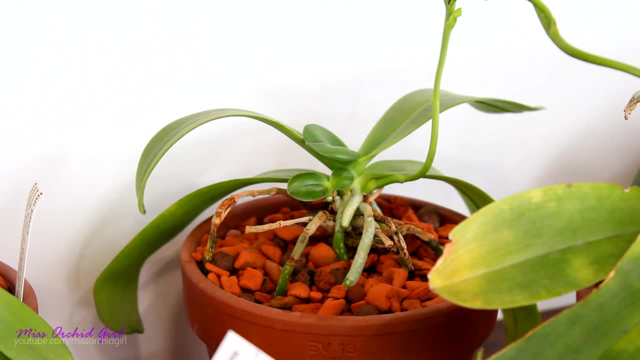 talk about what a caky is and how it differentiates from a new growth. I'll link you to that video in an info card and also down below so you can learn more. But to sum it all up, a caky is a baby plant produced by an existing mature plant and theoretically it is an exact copy of that. 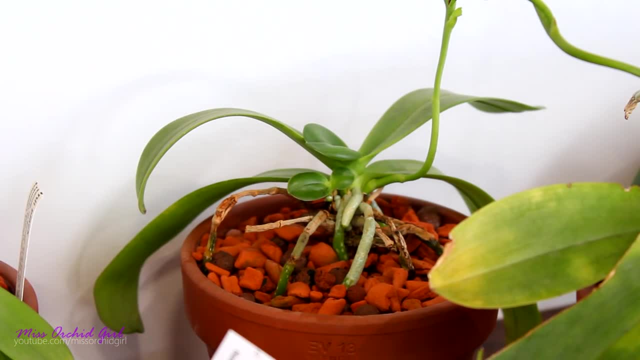 plant. Now, cakies are a means of propagation for the orchid, just like flower production. The difference between the two is that flower production refers more to the propagation of the species, while a caky refers to the propagation of an individual. Now I will debate a little more about this subject. 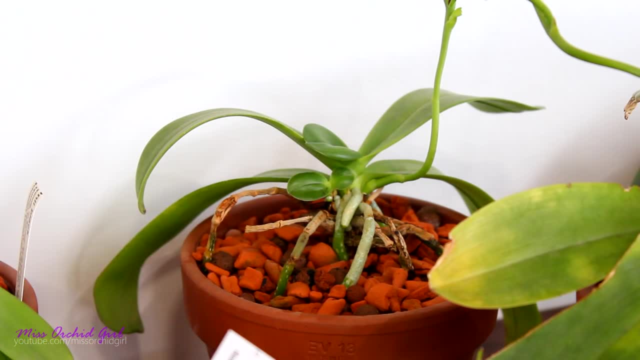 further on in the video. Let's just leave it at that right now. So that's what a caky is. And to answer to my viewer's question, since cakies are a way of propagation, yes, they can be produced in a. 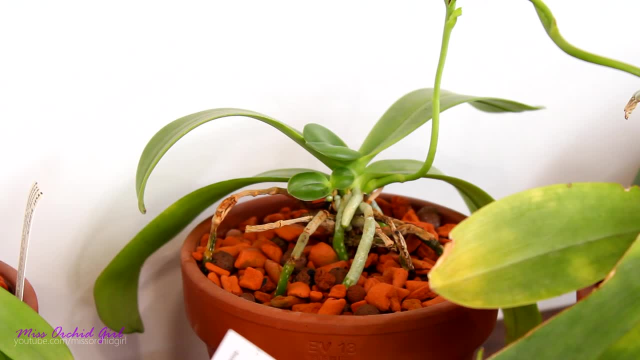 variety of ways. I'll give you three more situations in which orchids that are perfectly healthy can produce cakies without you stressing them or artificially intervening to determine the production of a caky. But to get to that we need to take some facts into account. So first of all, 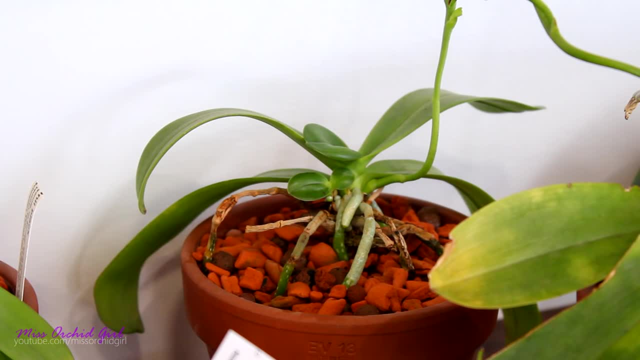 what actually determines the production of a caky? And to answer that, I'll give you the most non-scientific explanation ever, just so you can see that you don't really need heavy biology knowledge. just to put two and two together. Now, if you are in the hobby for a little while, 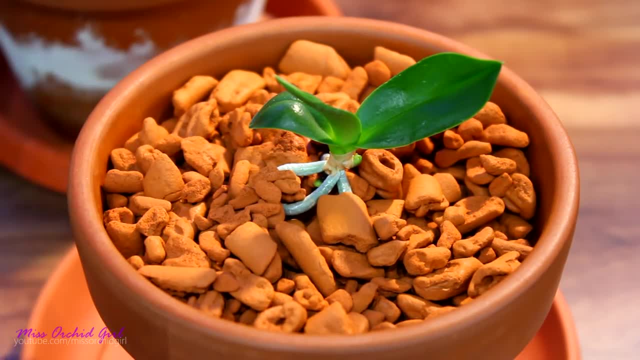 you might have already heard of the famous product called caky paste. What it is, it's a gooey substance that you place at one of the growth nodes of an orchid. We'll get to that later And if you wish really hard, a caky will sprout from that node. If you dig a little bit more and see what. 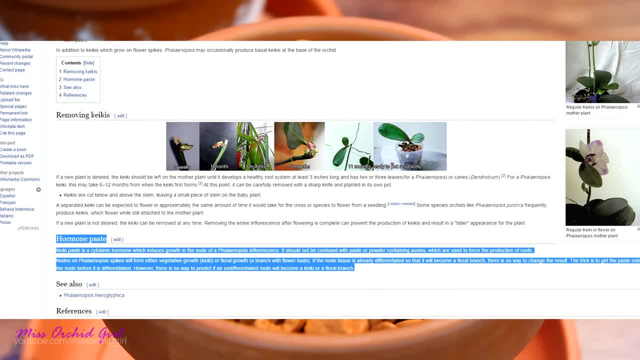 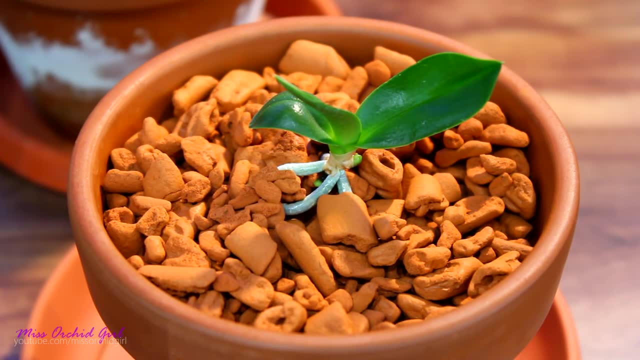 exactly caky paste is, you will discover it is actually a growth hormone or it actually contains a growth hormone, specifically cytokinin. Thus, we can safely assume that hormones have something to do with the production of cakies. And yes, you are correct. So see, that was easy. I don't need heavy biology knowledge, But we can. 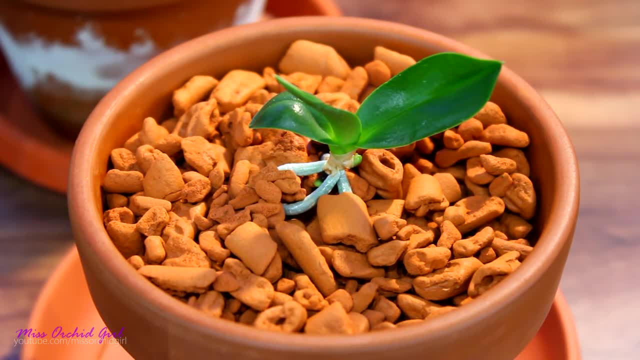 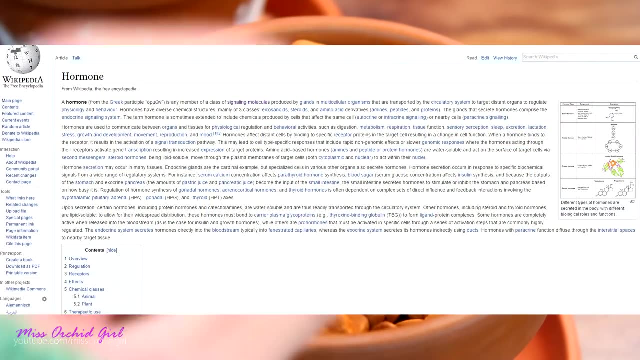 also take this further so we can better understand the process. Let's just take a look at what a hormone is. Now I will give you the general definition of hormones, because the definition of a plant hormone lacks a certain part, And to translate this into orchid talk, a hormone is a. 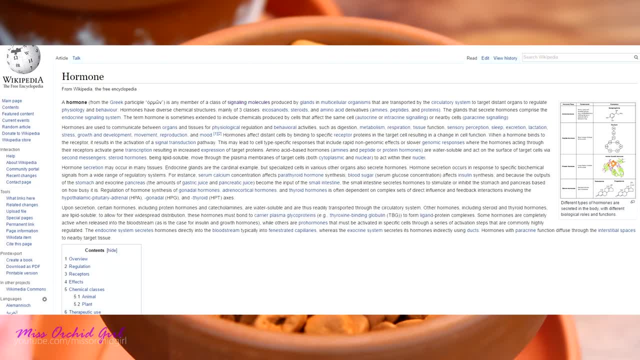 cell produced by the orchid that is directed at different structures, such as growth nodes, and has the ability to dictate what those growth nodes can do. Now, cytokinin is a cell produced by the orchid that is directed at different structures, such as growth nodes, and has the ability to dictate what those growth nodes can do. Now, cytokinin is a 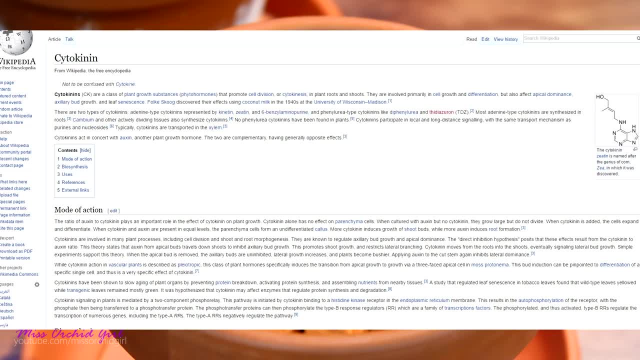 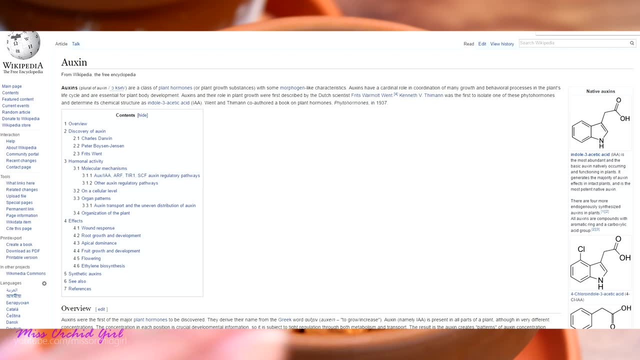 hormone responsible with cell division, but it's not the only hormone that plants and orchids have. Another important hormone is auxin, So within an orchid we always have a certain ratio. Sometimes one of the hormones might be at a lower level and the other one at a higher level, and vice versa. 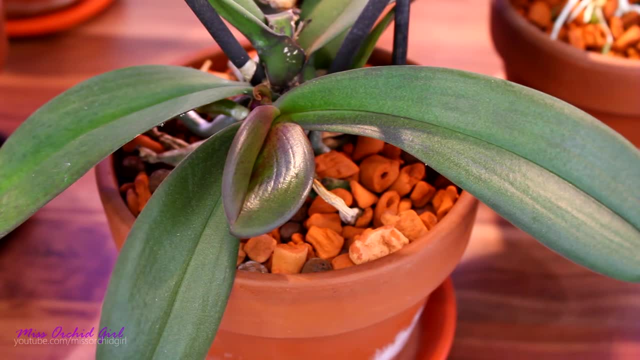 Now, the most prone orchids that produce cakies are monopodial orchids, such as Phalaenopsis, Vanda orchids, Angraecums, Renaltheras and so on, But some sympodial orchids are capable of producing. cakies as well, things like dendrobiums or epidendrums, And even if they are two different types of orchids, they do have one thing in common, and that is the availability and number of nodes. So let's take the example of monopodial orchids. The growth nodes are situated on their stem. 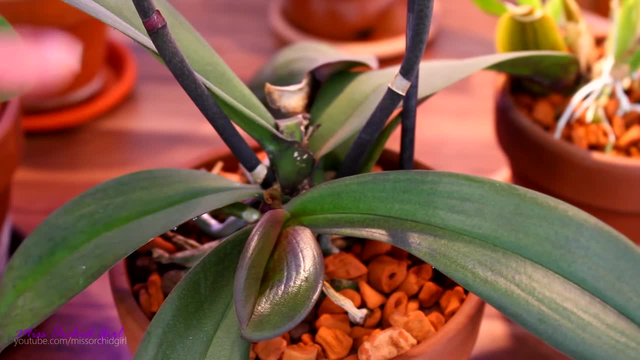 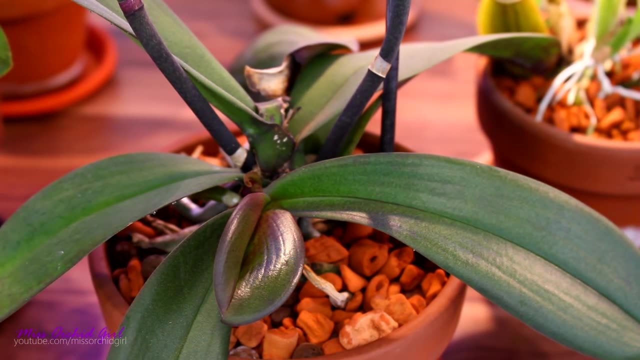 As you can see on the stem, leaves are produced, flower spikes are produced, but also cakies can be produced. What determines what structure will be produced? Well, it's this ratio and balance of hormones. Now, Phalaenopsis are a little bit different than other monopodials in the sense. 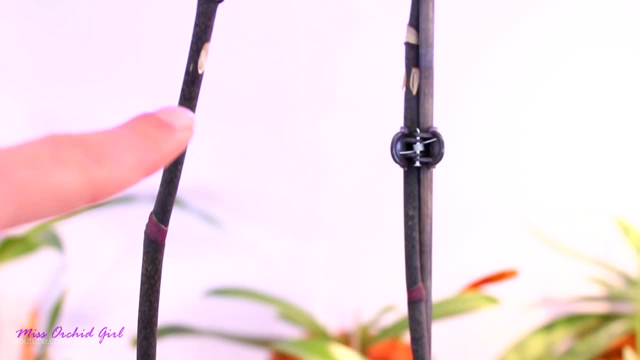 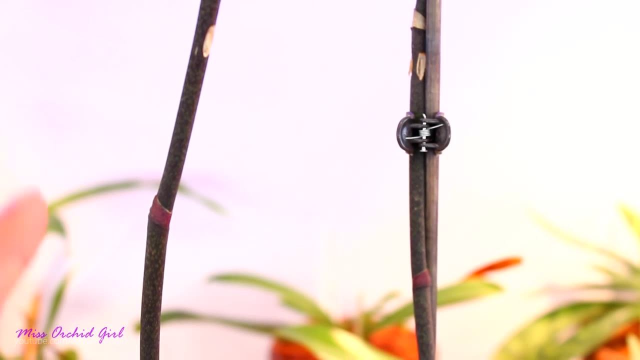 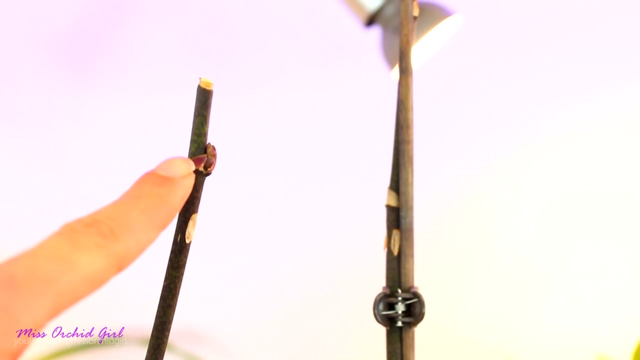 that they have growth nodes along their flower spikes as well, And the growth nodes are these structures that you can see here. We call them dormant buds or dormant eyes. Things can sprout from this node, such as a branch of a flower spike and even a cakie, Other monopodial orchids. 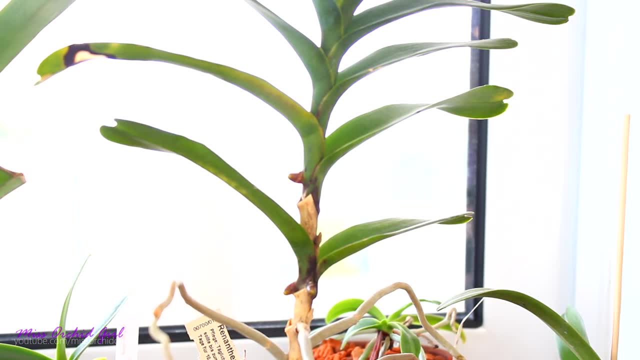 even if they don't have these growth nodes on their flower spikes, are similar to Phalaenopsis in the sense that they have growth nodes along their stem, in between the leaves. They can produce roots. Phalaenopsis can produce roots as well, They can produce cakies and they also can produce flower. 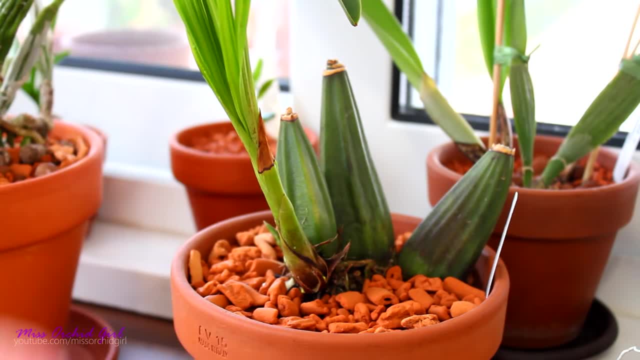 spikes. Now, yesterday we discussed about pseudobulbs and what they are, and we learned that they are actually a stem of a plant, in our case, an orchid that is inflated. So even though a sympodial orchid has pseudobulbs, they actually are stems and they do have growth points as well. The difference is. 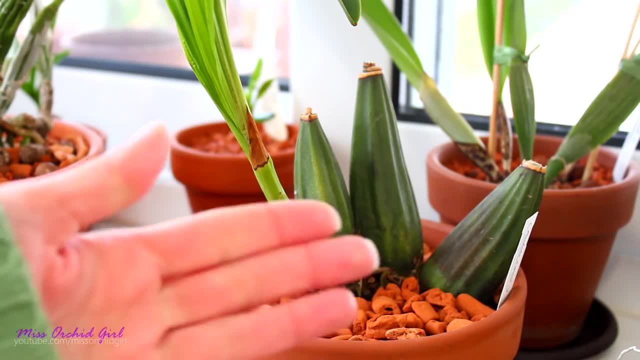 in this case, I don't have many growth nodes. I have only a few growth nodes. So I don't have many growth nodes, And if we take a look at these pseudobulbs, we can see that on the surface of a. 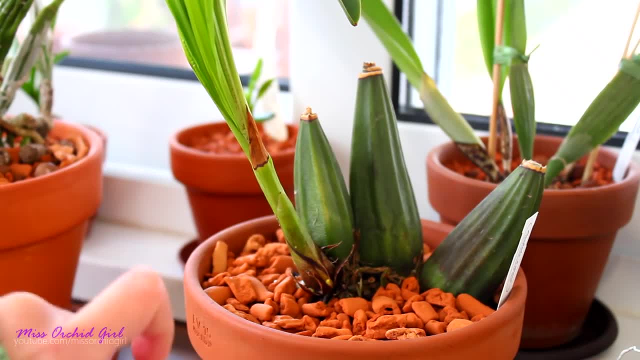 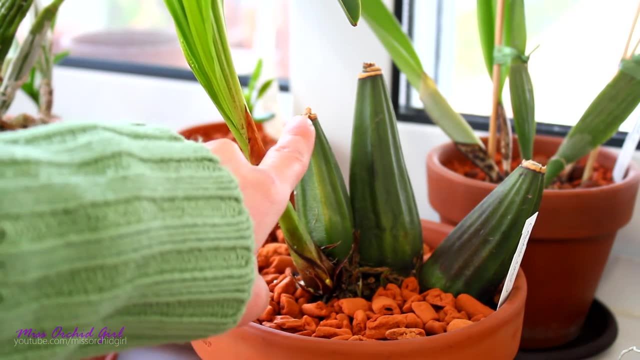 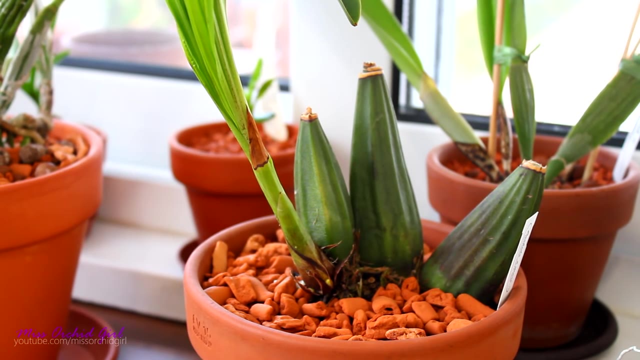 pseudobulb. we do not have any growth points. There are growth points at the base. They are responsible with the production of new growth or new pseudobulbs. And also we have growth points at the top because this is where leaves are growing. In some very rare cases, orchids like Oncidiums and 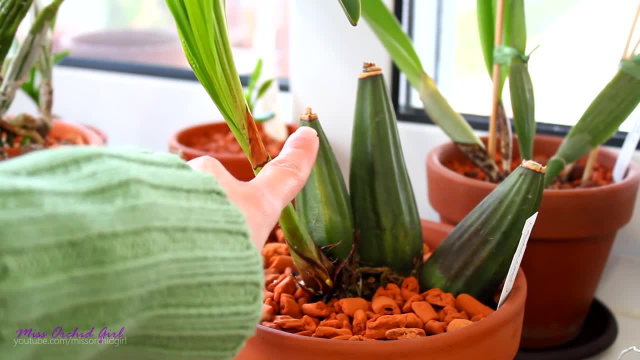 even Catleas can produce a cakie at the top of a pseudobulb because there is that growth node up there, But generally speaking it's not the case. In some very rare cases, orchids like Oncidiums and 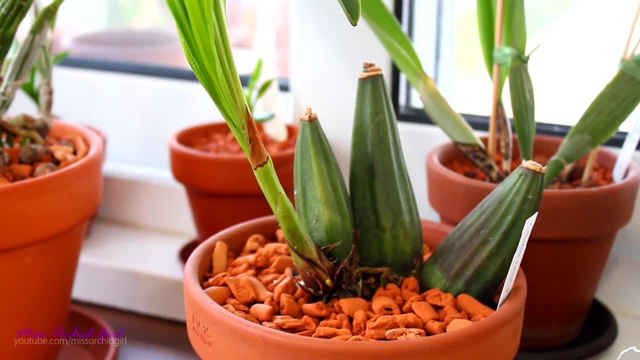 even Catleas can produce a cakie at the top of a pseudobulb, because there is that growth node up there, But generally speaking, they are not prone to producing cakies And in the vast majority of cases you will not have cakies on these orchids. On the other hand, things like Vendrobiums- 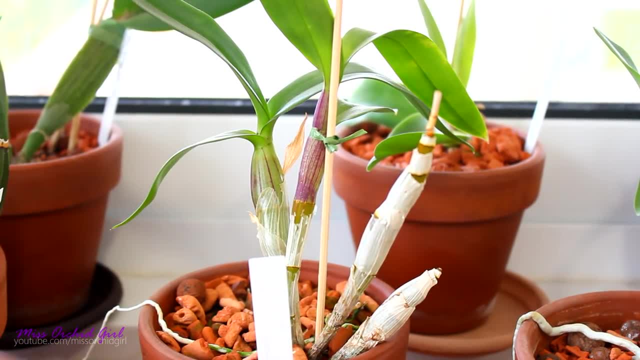 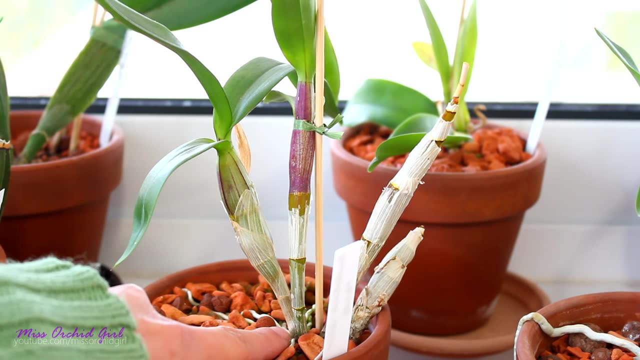 even though they have pseudobulbs. they have multiple nodes on the pseudobulb And this is a little bit more obvious than I know. but let's take a Phalaenopsis type Vendrobium. We have growth nodes at the base and they're responsible with creating the new growth or the new pseudobulb. 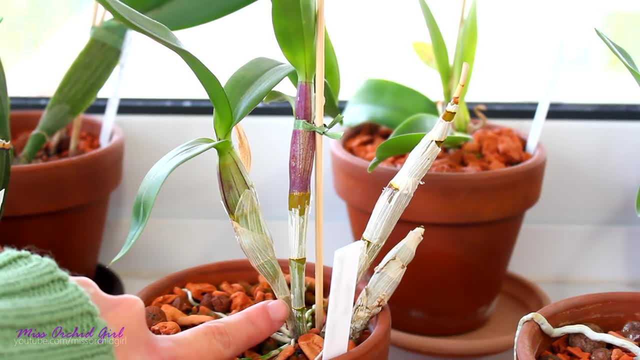 But also along the cane. we have multiple growth points. We have one here, one here, one here and one at the top. And even though some leaves are not present on my Vendrobium Phalaenopsis at the moment, the sheaths actually correspond to the leaves this orchid had. 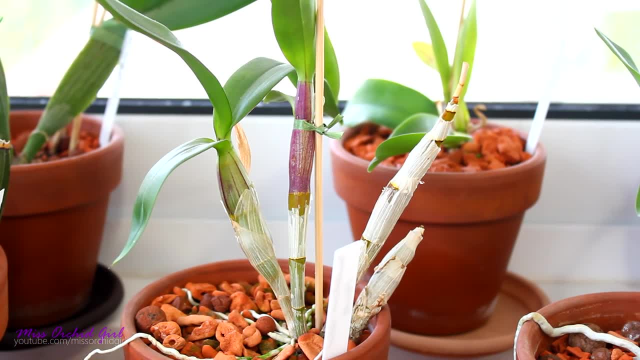 Now Vendrobiums, just like Epidendrums, can produce flower spikes from any of these nodes. But not only are flower spikes produced. cakies can be produced as well, Unlike Oncidiums and Catleas. 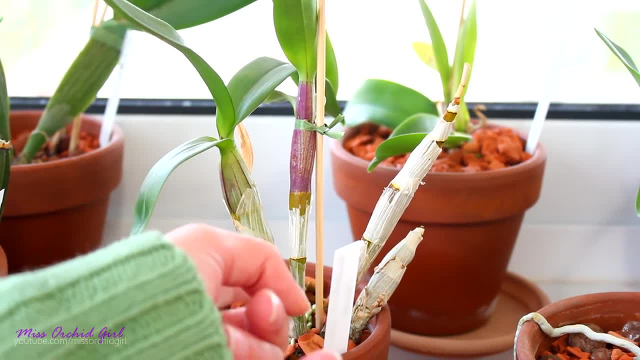 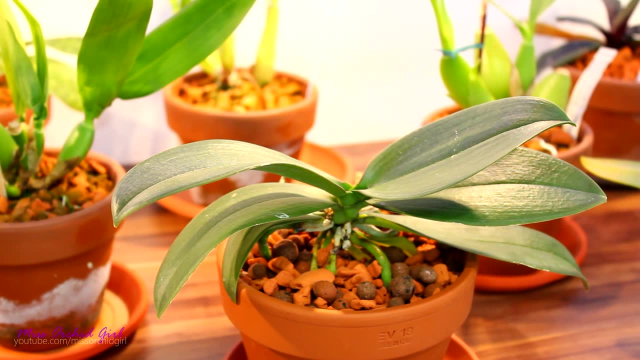 simply because there are more nodes and more growth points on the stem. these types of orchids are more prone to creating cakies, Then Oncidiums and Catleas. So, to sum it all up, the one responsible for the production of cakies. 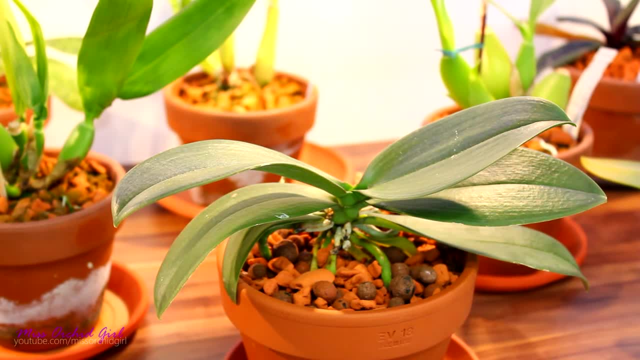 is the hormonal balance at the growth point or the eye, And this is how caky paste works. It provides a particular hormone at one of the growth points of the orchid. Now if you've ever experienced with caky paste, you know it's not 100% efficient in the sense that 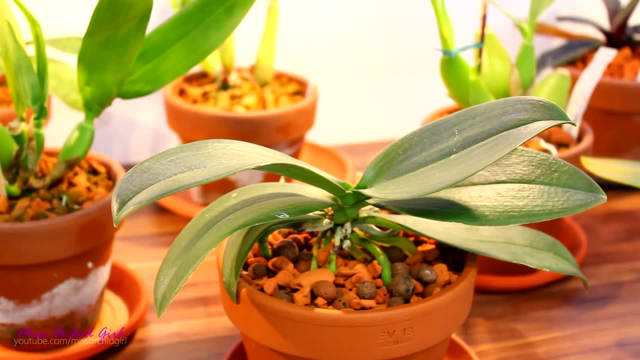 you can totally get flower spikes instead of cakies. Why does this happen? Well, it's because it already has a certain hormonal balance in that growth point And there is a chance that the hormone provided by the caky paste works in contradiction with the existing hormonal balance. 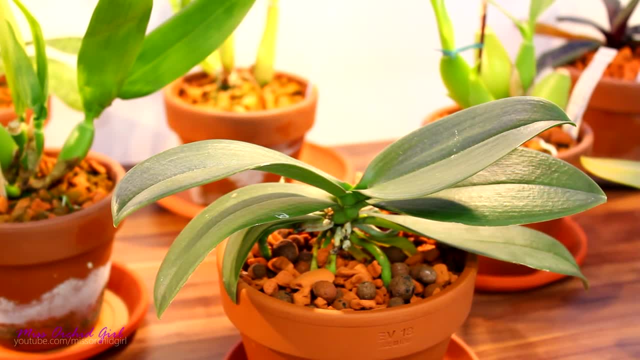 at that point, And since it's not an exact science, it all depends on the orchid you're applying caky paste to and its hormonal balance. Furthermore, an incorrect hormonal balance can lead to serious mutations or structures that are not viable, And I don't have a video to show you but Boutran here. 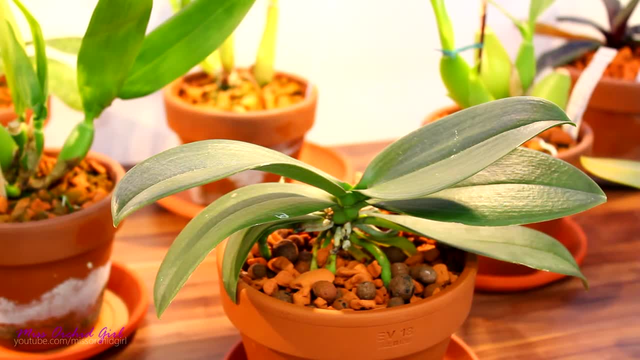 has a video. If I find it, I will link you down below to that video. She tried caky paste and the result was quite scary, in the sense that the flower spikes produced were really mutated, really mangled, And this is pretty much what happens when you're trying to play with hormones. 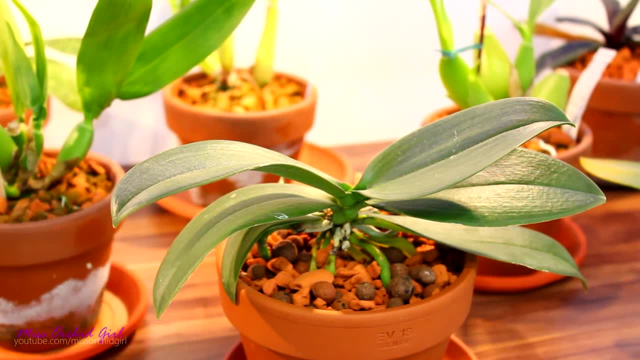 You can get some pretty awful anomalies, since hormones are responsible with creation and development of structures Inside the plant. there is a certain type of balance when it comes to hormones, And when we start to mess around with them, we can have some really weird results. 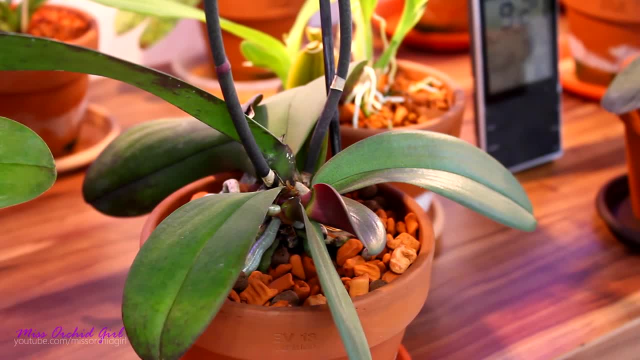 Alrighty, so this was the more factual part of the video. You have links to some articles down below. You can check them out and you can research further. And now let's get to a more theoretical approach to things and try to answer the question of why orchids produce cakies. So I was telling 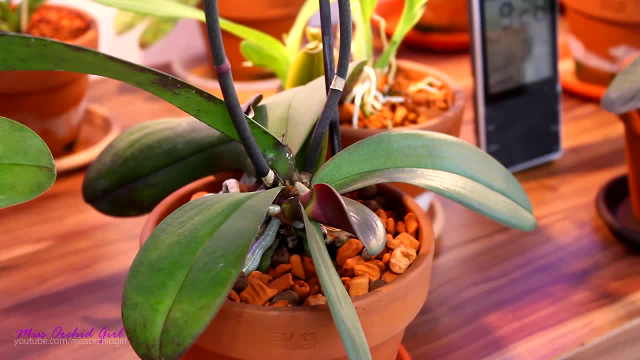 you that I have three instances in which orchids can produce cakies without you intervening artificially with caky paste or without you stressing the orchids. So first case: a perfectly healthy and vigorous orchid that you are growing in perfectly optimally. 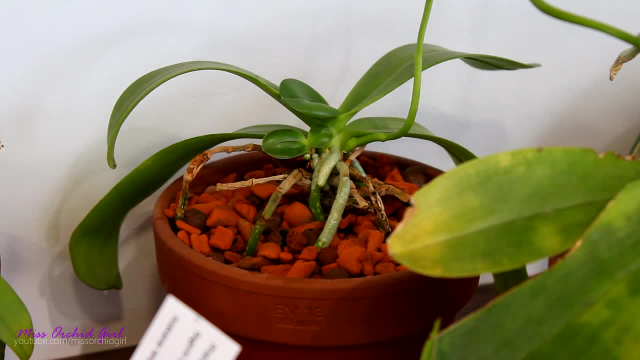 It can produce a caky. So to answer to the question of why this type of orchid produces cakies, we need to formulate some theories. So at the beginning of the video I was telling you that a caky is a way of propagating the individual orchid, not necessarily the species. What I 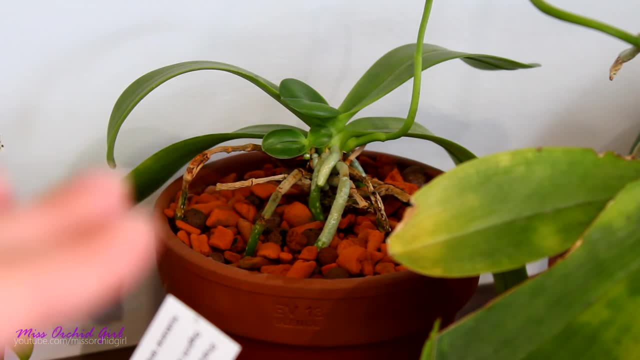 mean by this is that the structure responsible with propagation of the species is the flower. What makes it the most important propagation organ? Well, simply because of gene diversity In nature, it is really important to have diverse genes, And some plants go as far as to not accept pollen from their own flowers. 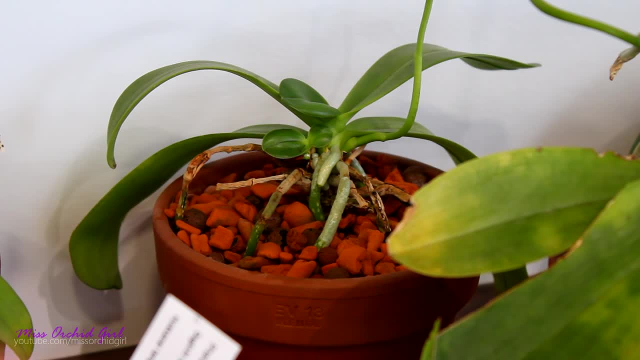 in order to produce seeds, but accept the pollen that comes from a different plant from the same species, but a totally different plant. Now, this is a way of adaptation. Not all plants and all orchids prefer this, but by gene diversity, they ensure that the next generation has a different. 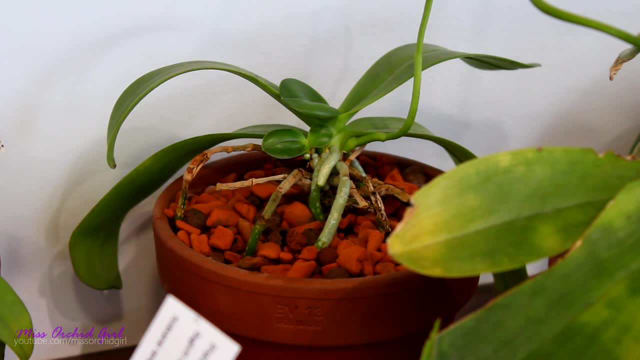 gene structure. Why is that helpful? Well, in a world of ever-changing and ever-evolving pathogens, plants and orchids need to ever change and ever adapt as well. If a plant only relies on cloning, it will have less chances to adapt to certain pathogens and even certain conditions that might. 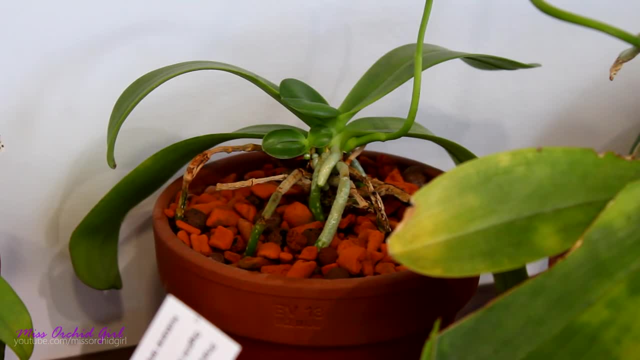 change in its environment over time. So, in my opinion, pollinization is the most efficient way of ensuring gene diversity. And by this I don't mean a certain orchid can pollinate a totally different orchid, resulting in a hybrid with special powers, No, it can be the very same species. 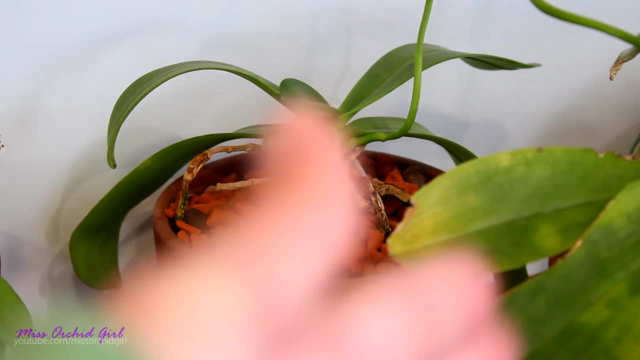 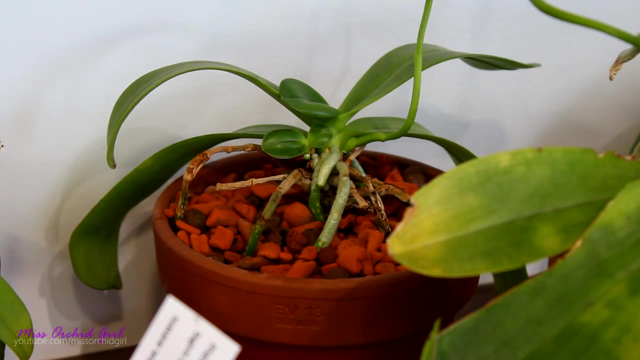 but one orchid is never identical with another orchid, even if they belong to the same genus. Now, as I was saying, theoretically a keiki is a clone of the same mother plant, And this kind of goes against gene diversity, doesn't it? Well, there might be a different purpose for that keiki. 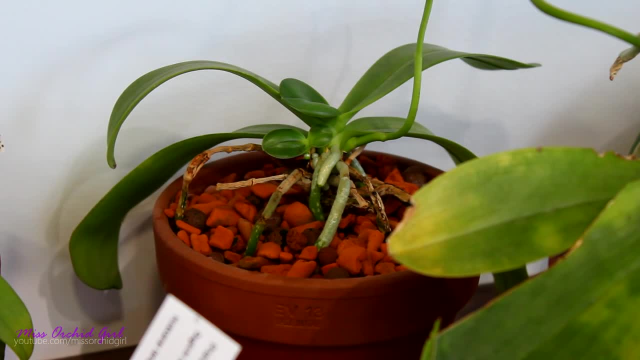 So, as you might know, an orchid takes a long, long, long time to develop from a seed to a mature and flowering size, And we are talking about years here. It can take 10 years, 15 years, even Now. 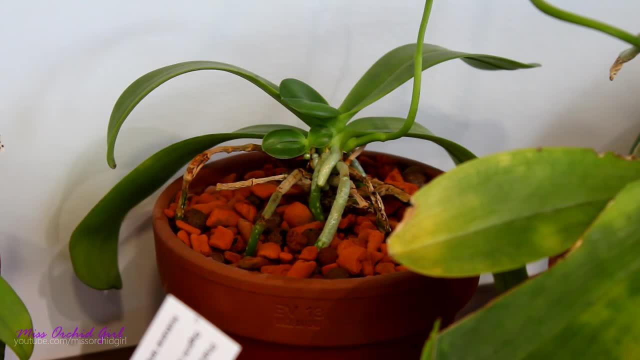 if an orchid takes that amount of time and actually reaches a size in which it is capable to produce keikis, some requirements need to be met. One: it needs to have a perfect location, whether we are talking about epiphytic orchids and their location on the tree. 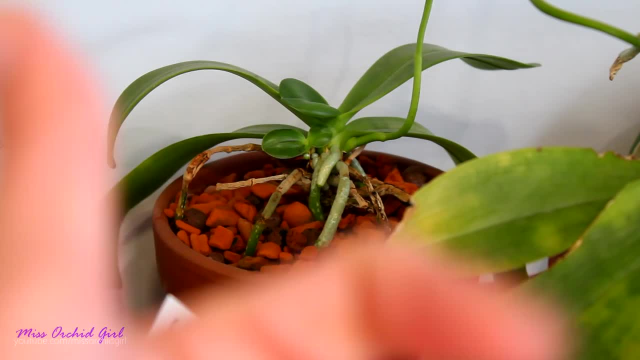 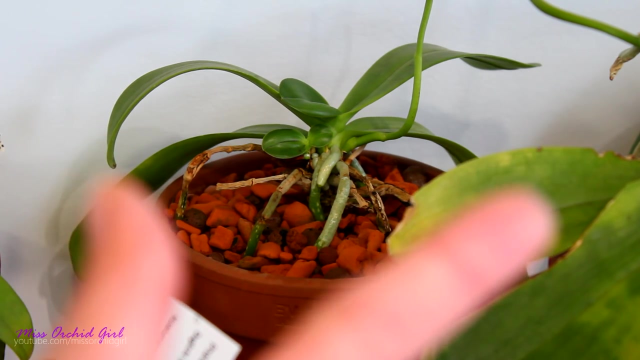 or terrestrial orchids and their location in the field. let's say They also must be very fit individuals to endure certain pathogens they might encounter until they reach maturity, And they also need to have a good gene pool to be able to reproduce. Overall this amount of time in which the orchid is alive can mean that that particular individual is one of the better individuals of the species. Now, through natural selection, only the best survive. And since this orchid survived, it would be logical for the orchid to produce even more flowers than it already does. And how does it do that? Well, it will grow a clone of itself. that. 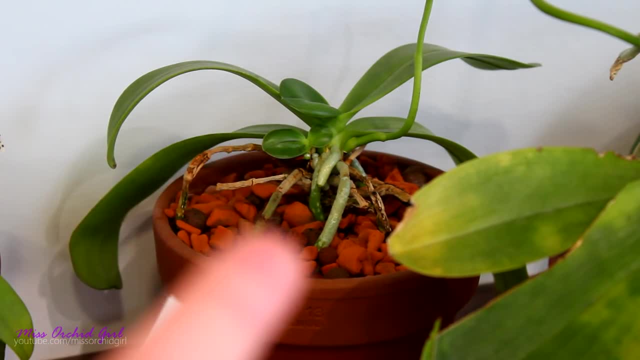 will be in the exact same location and will also share the gene pool of its mother orchid. When the keiki will start to bloom, this particular individual will not have, let's say, 10 blooms. it will have 20 blooms. Therefore. 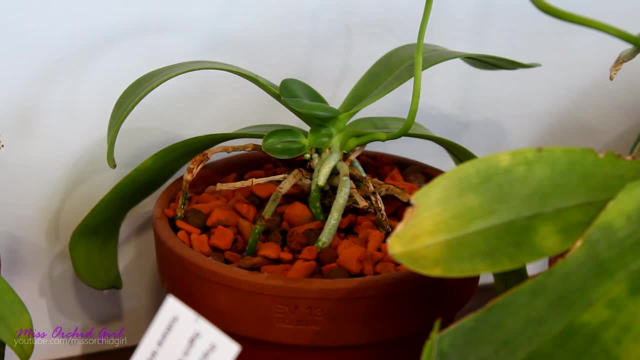 more chances of propagating the species through seeds. So for this reason I was saying that a keiki is a means of propagation of the individual and not necessarily a means of propagation of the species. But in this case it is perfectly possible for an orchid that is very healthy and very 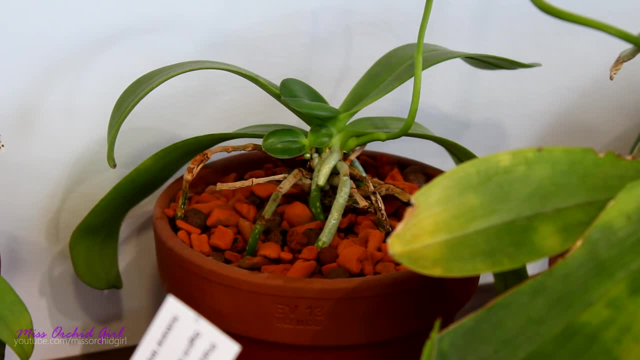 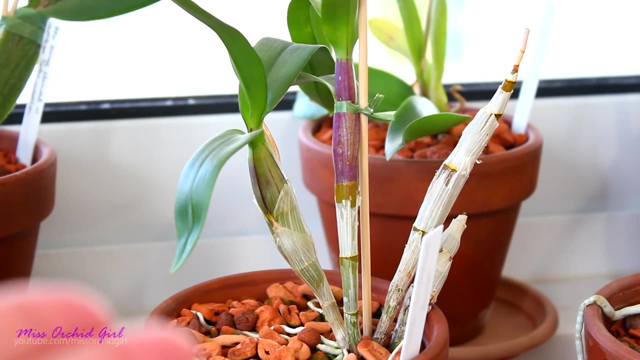 vigorous and has a perfect location to try and replicate itself. so it has more chances to get propagated Now. second instance: a perfectly healthy orchid produces keikis because of external factors. And yes, the hormonal balance can totally be affected by external factors. 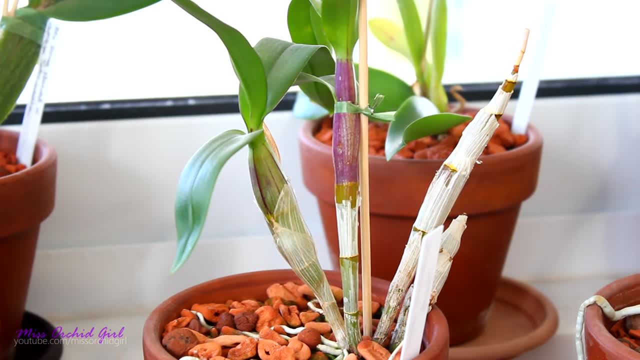 as they actually induce a certain chemistry on the orchid, And I'll give you the example of certain dendrobiums: Things like the kingianum and even the nobilis are more prone to producing keikis if conditions are very warm, if water is provided and 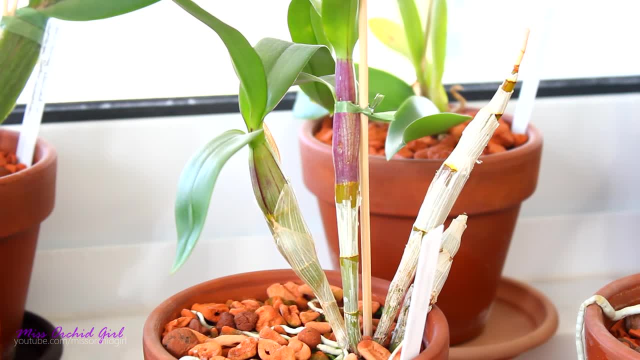 fertilizer is provided as well. Usually they will produce better flowering if temperatures erupt, if water is reduced and fertilizer is cut altogether. Now, because this is not an exact science, some orchids may tolerate not ideal conditions. let's call it like that: better than. 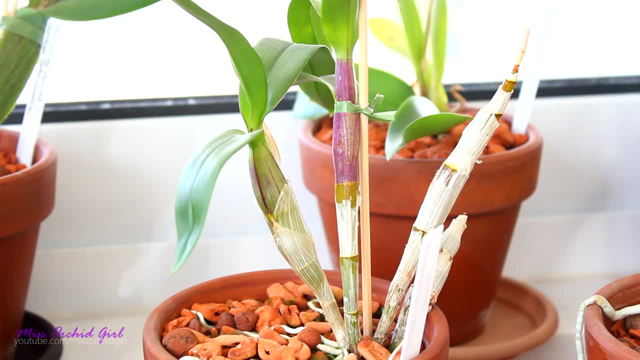 others and they might flower without this change in environment, While for others the change in environment is totally necessary. Now some might debate that the change in environment, the lowering of temperatures and withhold of fertilizer is a type of stress. Certain external factors determine. 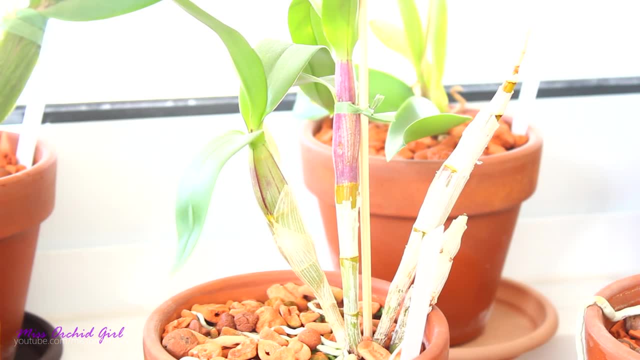 a certain chemistry and a certain hormonal balance. If it's too warm, the orchid might produce excessive cytokinin and therefore we will have an abundance of keikis rather than an abundance of flowers. So in this example, again, we cannot talk about a certain stress for the orchid. 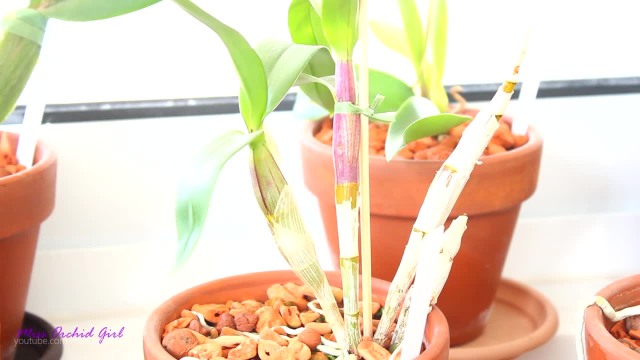 Moreover, we maintain temperatures normal and at a comfortable level, we offered fertilizer and we offered water, and all of these external factors determine the apparition of keikis, And I think this is the perfect counterexample to the idea that orchids are a type of stress, and they are a type of stress and they are a type of stress and they. 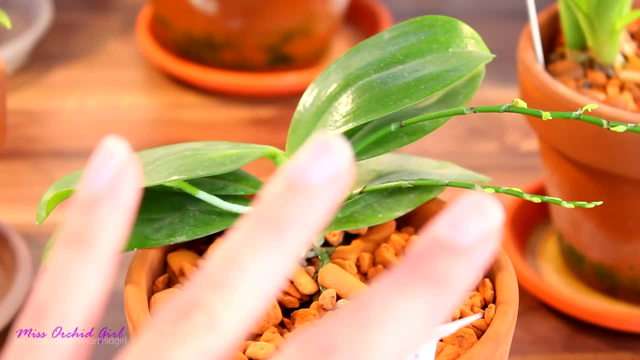 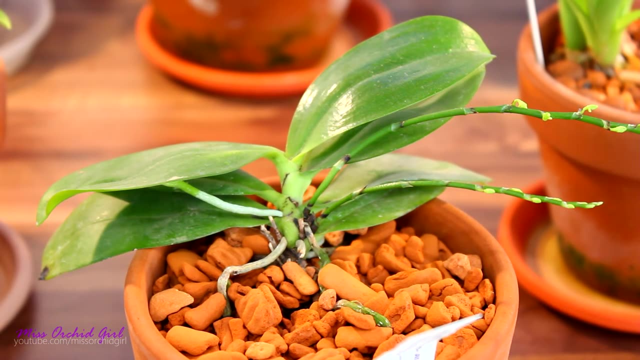 produce keikis because of stress. And the third example refers to a genetic anomaly. And this is a pretty elaborate discussion. I'll try to make it short, Because some of our orchids are super hybridized, some genes might have been lost or might have been messed with. And one example of 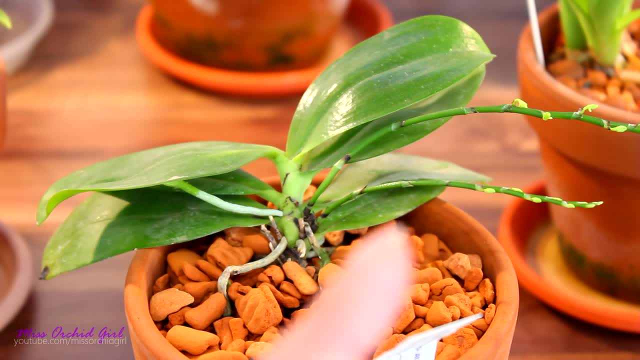 this sort of gene mix-up, which I consider to be the epiphany of hormonal imbalance, is the dendrobium stardust, which is absolutely prone to creating keikis excessively. Both of my stardust dendrobiums were lost due to excessive keikis and I'm not exaggerating: On one of them I counted. 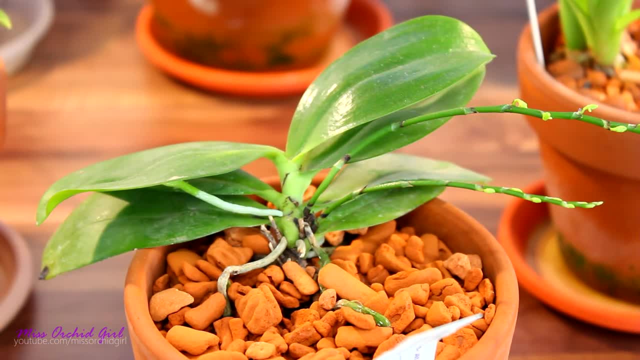 30. And other growers have the same problem with this particular hybrid. How did this happen? Well, if you search the parentage of this dendrobium, you will find that we have the dendrobium unicum, which is a species, as a parent, And the unicum is known to produce quite a lot of flowers. If we take 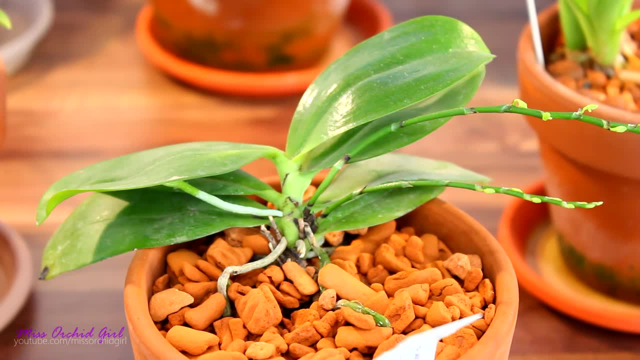 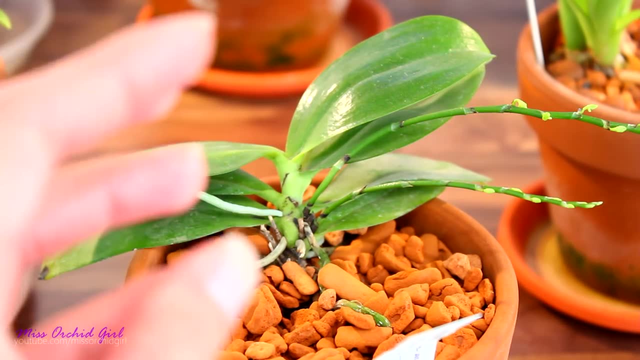 a look at the other parent, you can see that one is a complex hybrid. So, theoretically, if you mix an orchid which would produce a lot of flowers, you would have a complex hybrid. And if you mix an orchid which produces an abundance of flowers and not so many keikis and you mix it with an, 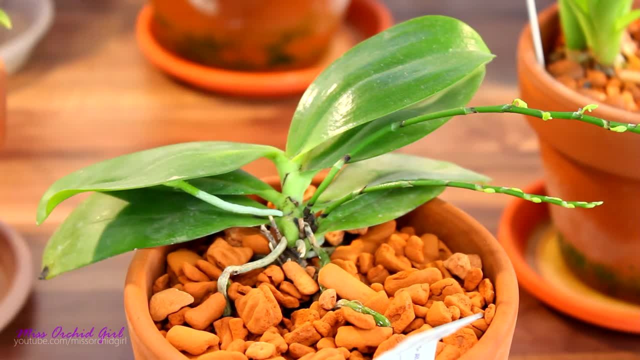 orchid that produces one or two flowers and actually produces quite a lot of keikis. due to its nature, you might end up with a hybrid that produces an abundance of flowers and also an abundance of keikis, And that's never a good combination. The flower production takes a lot. 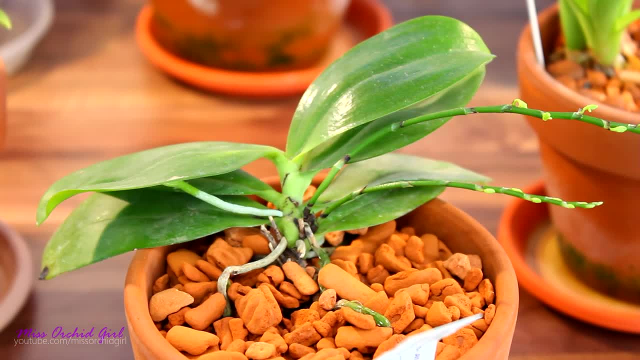 of energy from the orchid. Keiki production takes even more energy from the orchid. You put them together and you spell this together, And if you mix an orchid with a dendrobium you get a disaster. Now these genetic anomalies are not that easy to see, Usually when we hybridize. 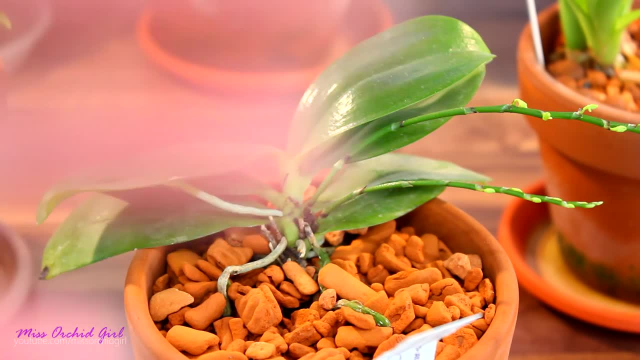 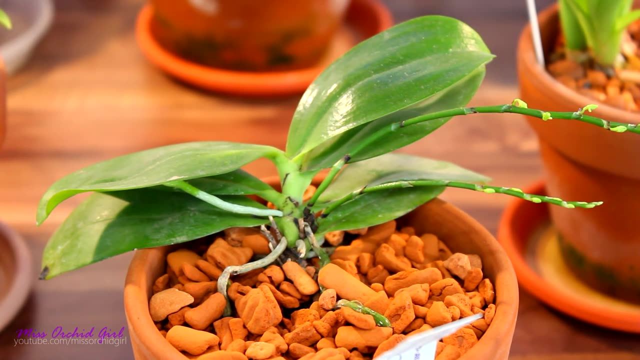 orchids, we are looking for visible anomalies such as deformed flowers or not very appealing flowers or deformed leaves or pseudobulbs, But when it comes to hormonal balance, this is pretty invisible to see. We take a look at the orchid, we find it looks pretty, has decent flowers and we 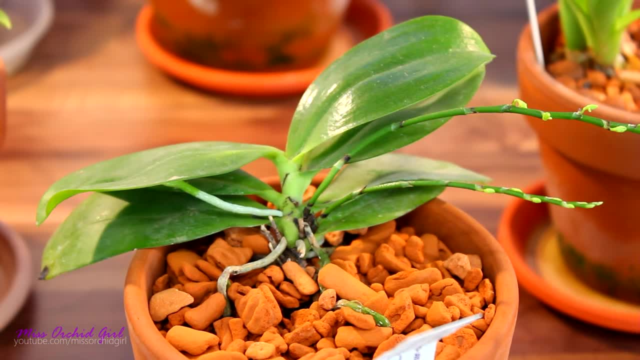 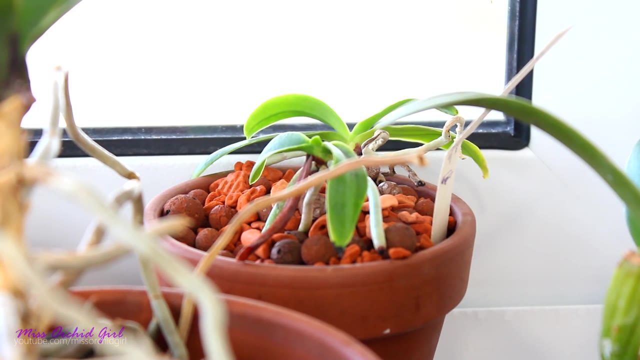 call it a success. But sometimes it just so happens that the genes split in such a way that the orchid has a very weird hormonal balance which makes it incapable of sustaining both flowers and keikis at the same time. But strictly speaking, the orchid is perfectly healthy. But this doesn't only happen. 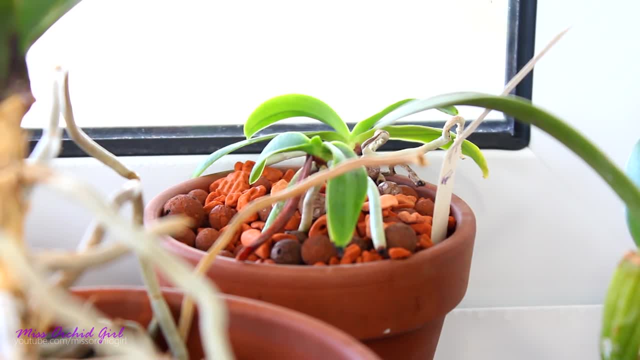 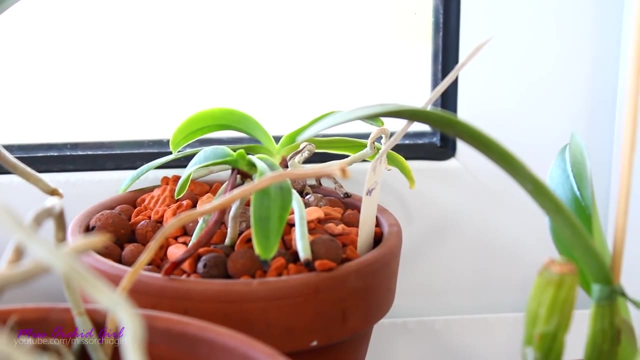 to hybrids. There are also species that we can own which are very prone to keikis, And I will remind you about my Cideria japonica. right there I have one which had four keikis and the orchid could not handle them, And one that grows normally no keikis. it bloomed, But this is a very weird. 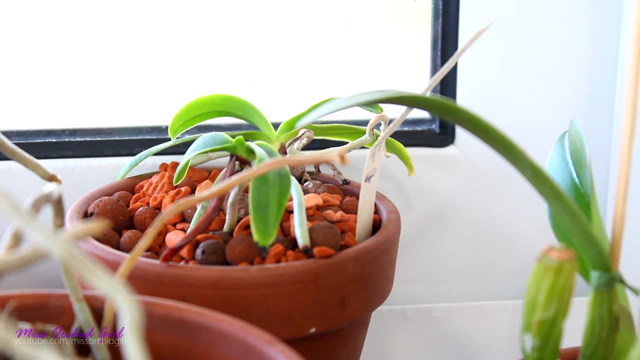 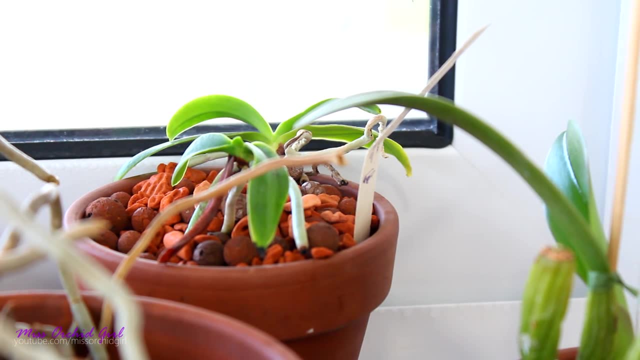 one. This one simply had this genetic anomaly to it. How does this happen, since it's not a hybrid? Well, through artificial propagation. we don't go through natural selection necessarily. We want quantity, don't we? And again, this anomaly is invisible. So we do take the individuals that look. 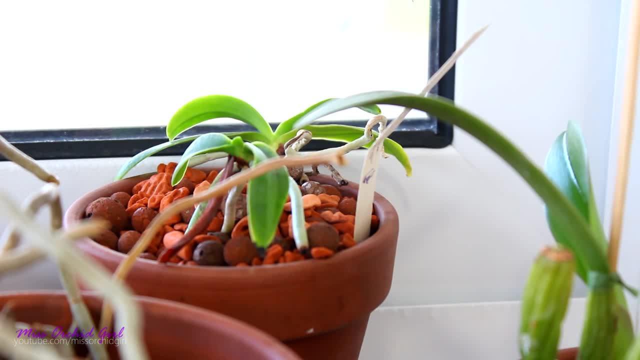 good. We offer the best conditions possible, so they all have a chance of survival. So the process in which we separate the non-fit orchids and the fit orchids is a little bit impaired when it comes to hormonal balance. Therefore, we can end up with an individual which is prone to creating 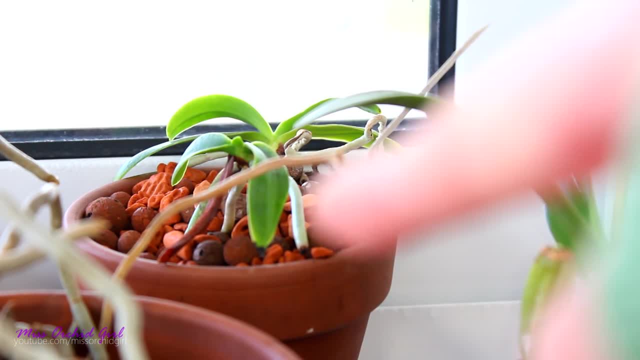 more keikis than it can sustain, such as that one over there. This, however, doesn't mean the orchid is sick in any way. It can be perfectly healthy And when it will start to produce a lot of keikis. 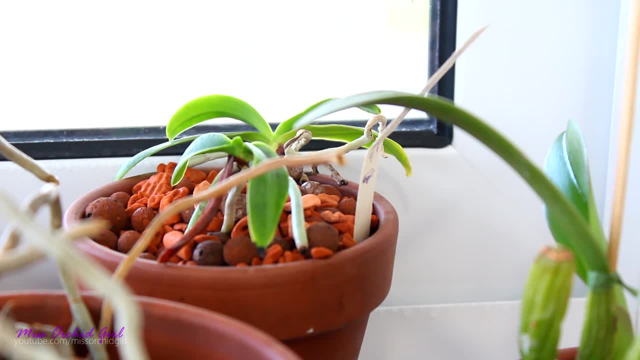 its health will demise, of course. But initially the orchid is perfectly healthy, It is kept in perfectly adequate conditions, It is fed, It is given light And all of that. you are not intervening artificially with keiki paste And still it creates an abundance of keikis. 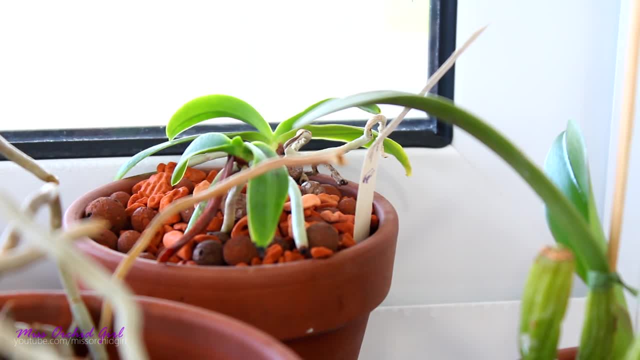 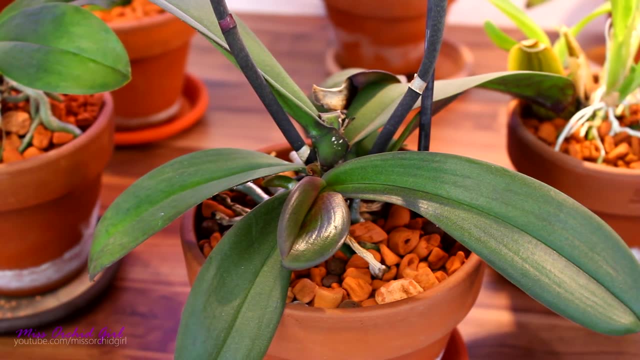 Even though the genus overall is not prone to creating keikis. So these were three instances in which perfectly healthy orchids produce keikis, But at the same time, keikis can be produced due to stress, And it's a well-known factor that if an orchid gets crown rot, it will try to remain. 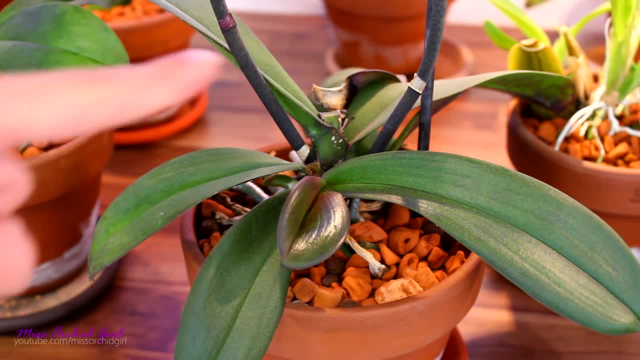 alive and propagate itself through keikis, either basal, either flower spike keikis. Now why would it do that? If it's sick, it means it's not a fit individual. Well, not really. The fact that an orchid gets crown rot it means it's not a fit individual. And if it's sick it means it's not a 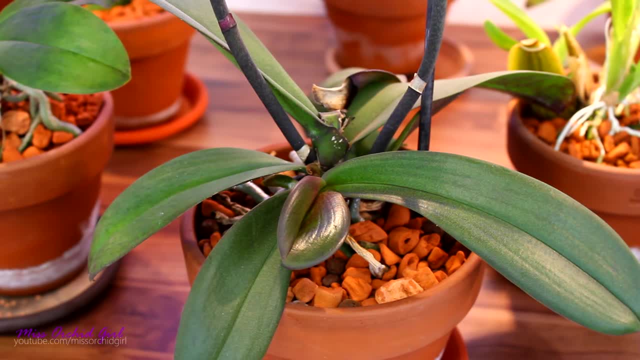 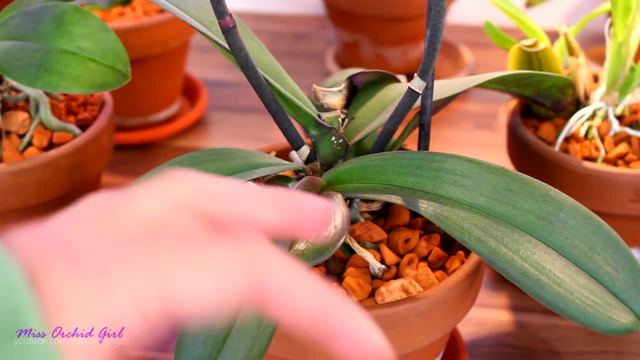 fit, individual, But nature doesn't necessarily mean it's not fit or that it doesn't have a good location to propagate itself and continue living. I'll give you a theoretical example. This orchid lived pretty well for 10 years And one day a leaf falls in its crown And it gets stuck there. 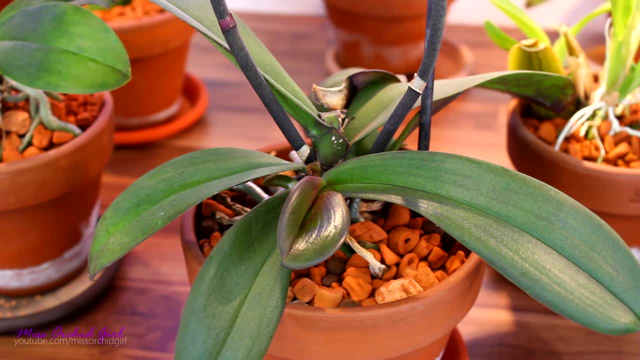 somehow The leaf starts to decompose, It maintains the crown moist, The abundance of bacteria starts to affect the crown of the orchid And the orchid develops crown rot. This is a very unlikely situation, But if one in a million happens, it's not a fit individual. And it's not a fit individual. 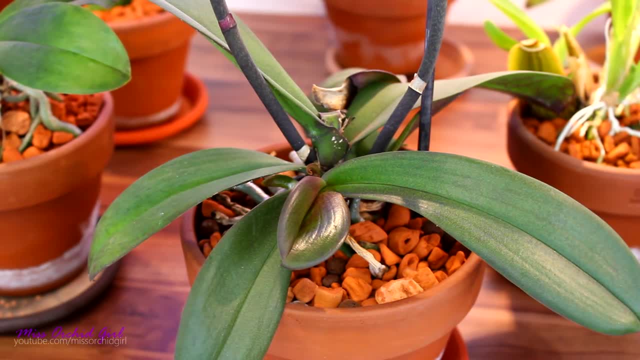 It is a variable And it doesn't mean the orchid isn't fit. Therefore it will try to continue its existence in the exact same place through the production of a keiki. So in this case, a true stress on the orchid determines a change in the hormonal balance of the orchid. So because she 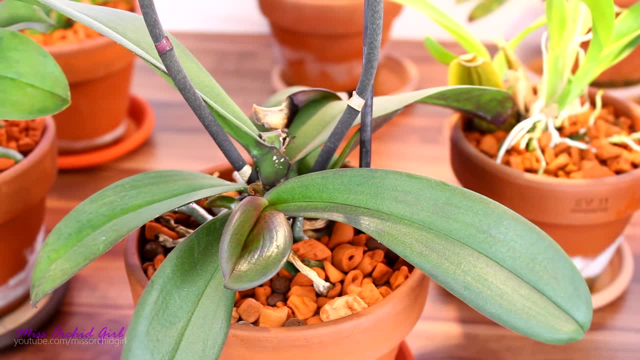 cannot focus her energy into new leaf production- and also the root system is totally fine. she does redirect all of her energy into the production of the keikis, which will carry on This particular individual, which by all means it is a perfectly fit individual that simply had a 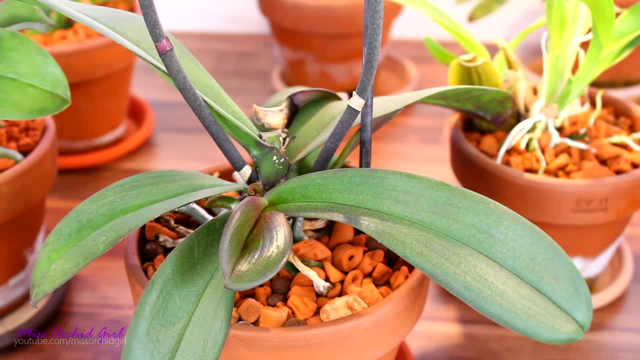 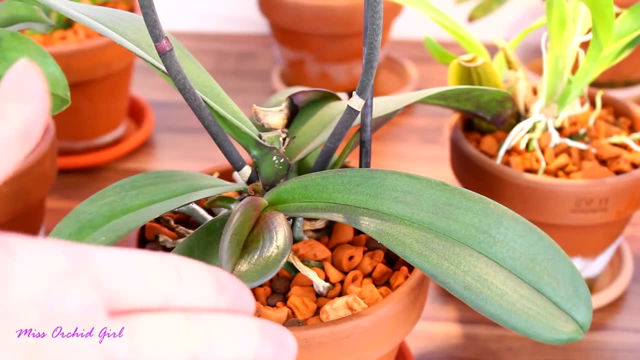 little bit of bad luck. So, from the evolutionary point of view of the orchid keikis, are a perfectly logical way to ensure that the individual itself propagates through the means of a clone. And of course the clone will have the same gene pool as the mother plant and will continue to produce. 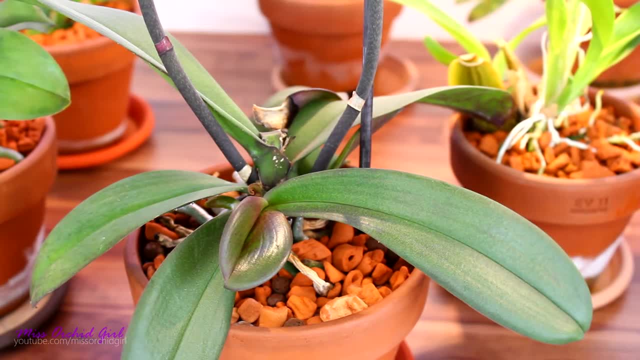 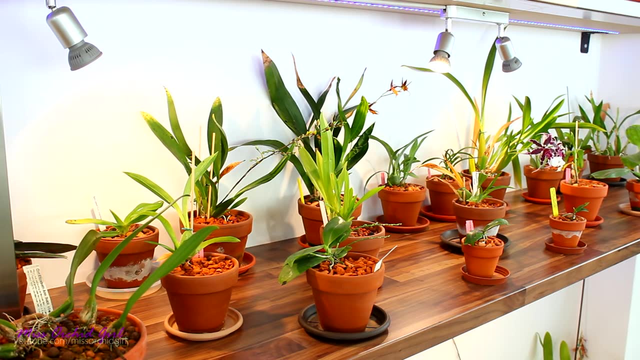 flowers and make its contribution to the propagation of the species. So overall I don't think keikis can only be produced in stressful situations. I think both perfectly healthy and happy orchids and also sick orchids are capable of producing keikis in 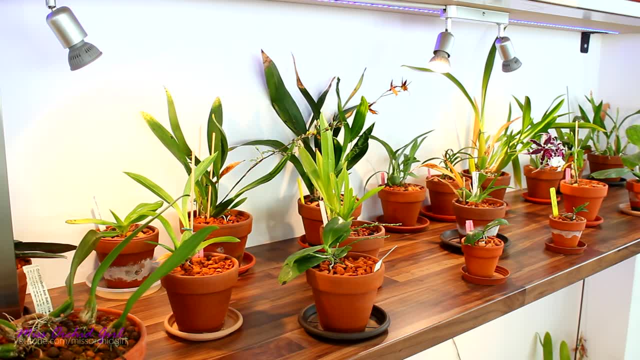 response to stress, in response to good conditions or simply as a consequence of this genetic pool. And that is my opinion on things. That is what makes sense to me, But, of course, if you have your own theories, let me know down below And, of course, if you have further articles for me to